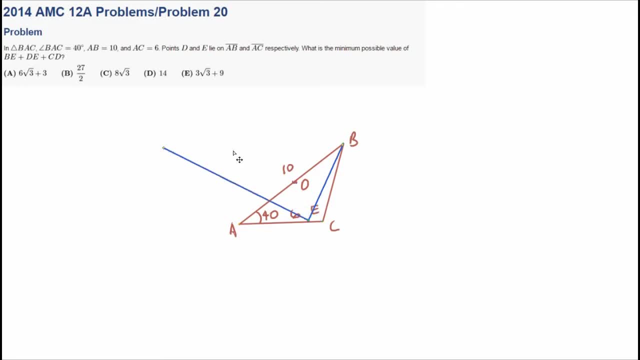 Okay, so for now, let's not get, let's not, Let's not draw that line so it won't get too messy, And let's reflect the shape across A, B. So let's see if I can copy this: 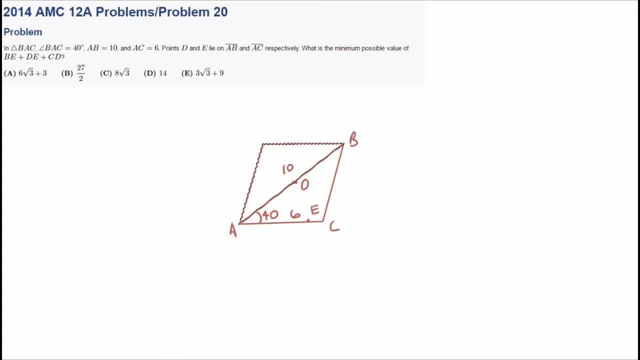 Okay, That's something. And then that's not the only time we're going to reflect it. We're going to reflect it again. How do I do this? Oh, I have to flip vertically, Reflect it again like this. You'll see why. 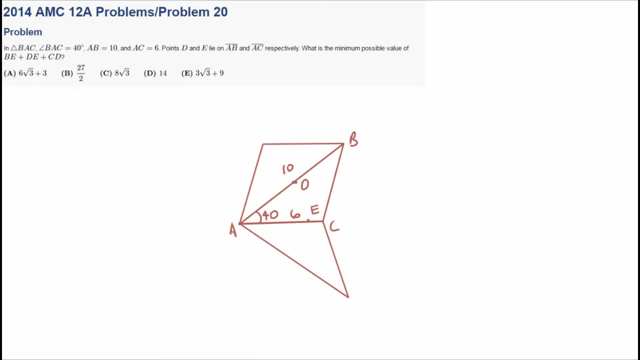 And one more time. Sorry, I'm just going to do that. So there you go. So we've reflected the shape quite a few times across A- B, And then we reflected that across A- C And we're going to see why. 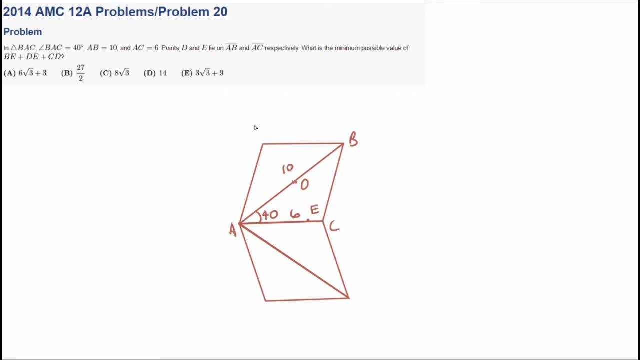 So that's A. Let's this be C. This is B1.. This is B, C2.. Because C is the obtuse angle of each of these triangles. Of course this is B2. But that won't matter very much. 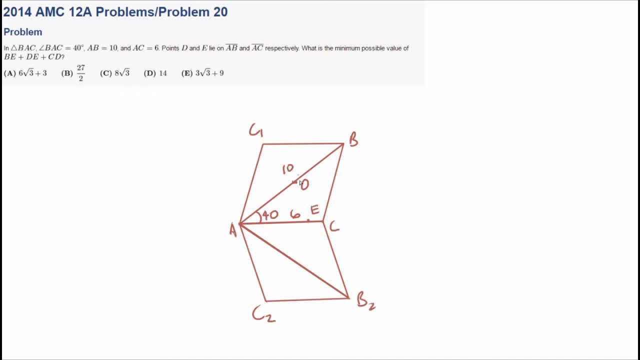 So what happens here? Let's draw D, Because you just reflect it across this, So it's D And E is still the same, And yeah, So that looks good. And let's try to see what exactly I did here. 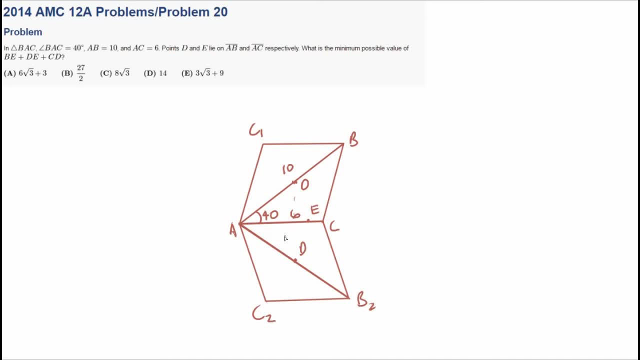 So we want to find the minimum possible value of essentially B? E plus D, E plus C, D, So B? E. is this Right? But instead of drawing the next line to D, Since the next portion, 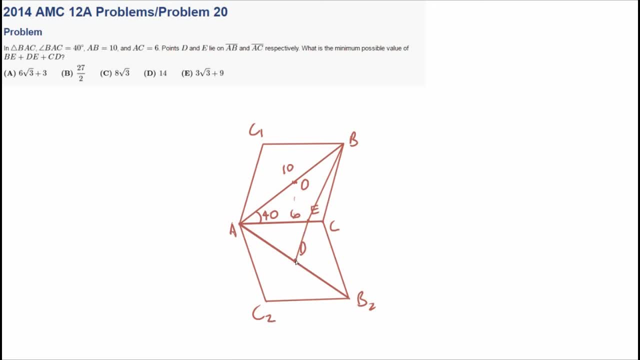 Is D? E. We're going to draw it to the second D Because, since it's reflected, The distance is equal, Right? So I should mark it down. This is D, D, D2,. I guess D2 is equal to D E. 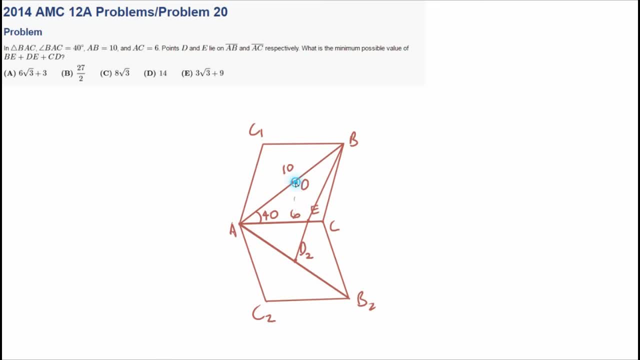 D2, E is equal to D- E, Because of course it's just a reflection. So this is just equal to this, And of course, the next one we're going to draw is from D to C, And instead of D to C, we're going to draw D2 to C2.. 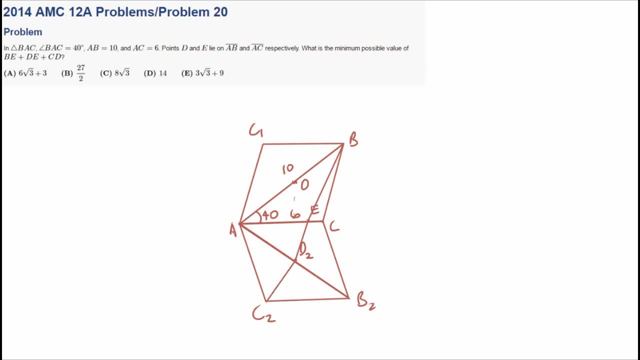 Because, since it's a reflection, D2 to C2 is essentially equal to D to C, Right, So D to C is equal to this And since this is a reflection, it's equal to this. Hopefully, you can see where I'm going here. 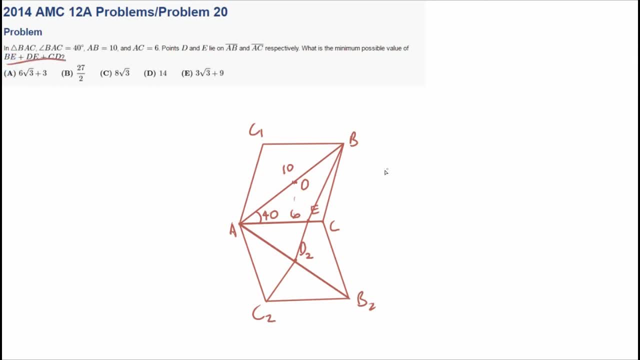 So essentially this quantity B? E plus D, E plus C, D is equal to B? E plus D2, E, Since it's a reflection Plus D2, C. So essentially you put down E and D such that you make a path between B and C2.. 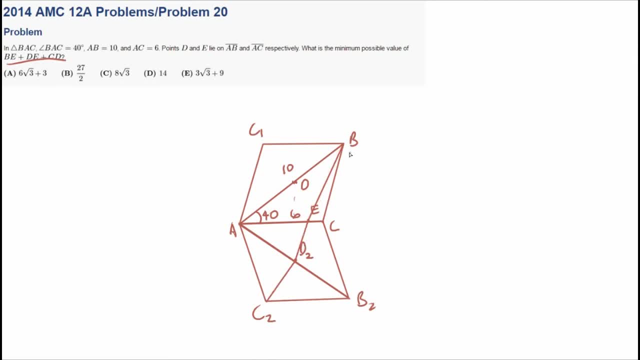 So there's a path between B and C2, right Along this path, And that's the distance. Well, the shortest path between B, B and C2 is just a straight line. And since you want to find the length of this path- the shortest length of this path, mind you. 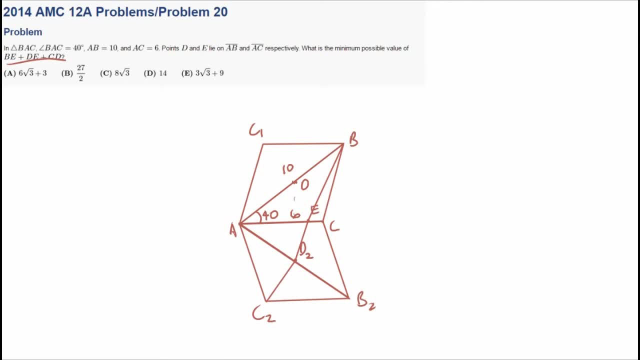 The shortest length of that path is just going to be a straight line. So actually, actually, what we want is, in order to find the shortest length, we want E to be actually right here and D to actually D2 to actually be right here. 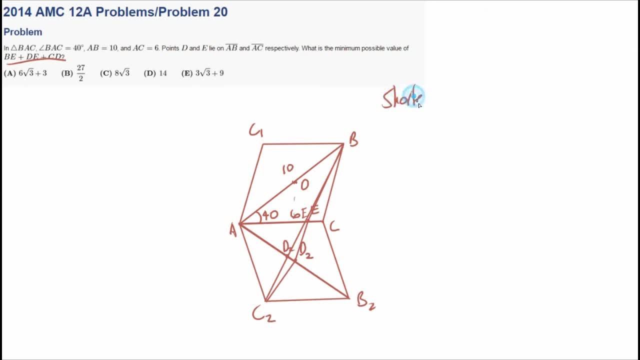 And the shortest path will just be B C D. So shortest path: B C D. Alright, And notice how we figured that out with reflections. So now, Now, how do I find this? How do I find this? the length of this path? 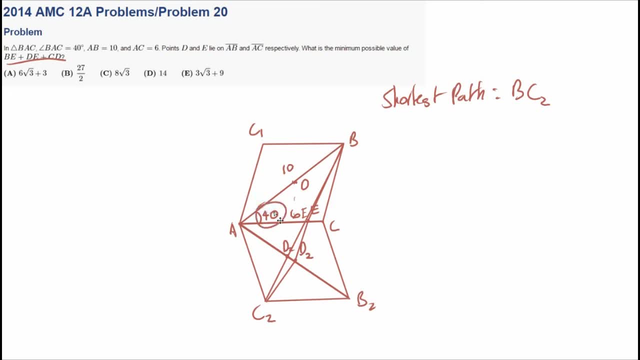 Well, actually it's not too hard, So notice how this angle is 40. We still haven't used that information yet, So 40.. Since the reflection of this angle is 40, right, And since this is also C2, A B2 is the reflection of C A B2.. 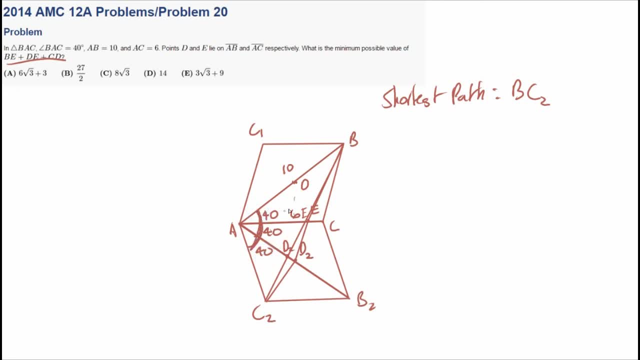 This is also 40. So totally, this angle, of course, is 120, right. The length of this is 10.. A- B is 10.. I see where you're going with this right. A- C is 6, right.